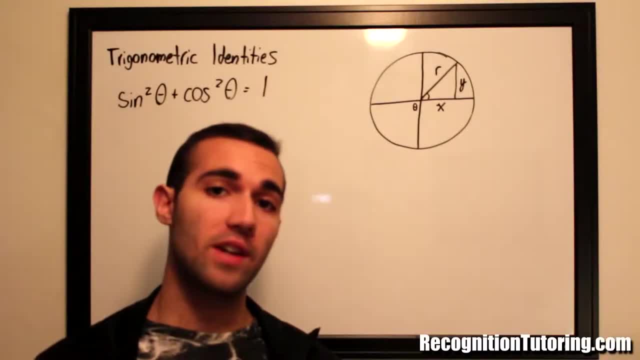 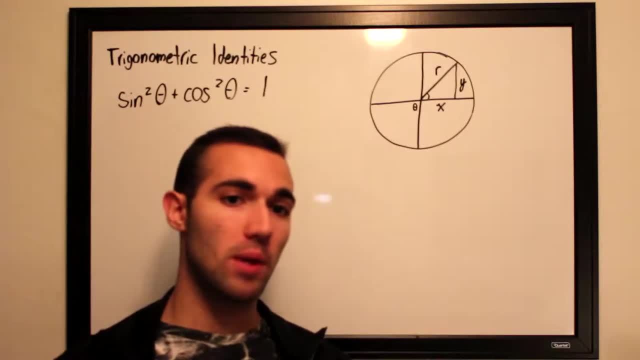 So in today's video, I'm going to be providing a very quick proof on why it is that sine squared theta plus cosine squared theta is equal to 1.. This is often a very common trigonometric identity that a lot of people don't- essentially don't know where it comes from, but it's something that it's expected to be memorized. 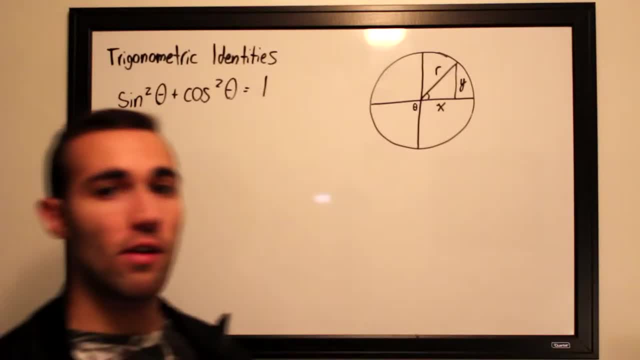 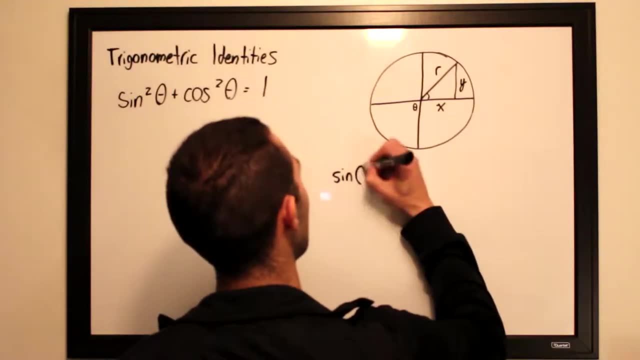 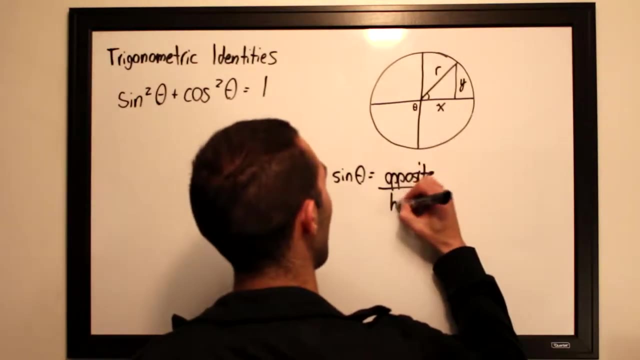 So here's a quick proof on that, using the unit circle. Now, very frequently we define the sine to be the opposite of a triangle divided by its hypotenuse. So the sine of theta is going to be equal to opposite divided by a hypotenuse. 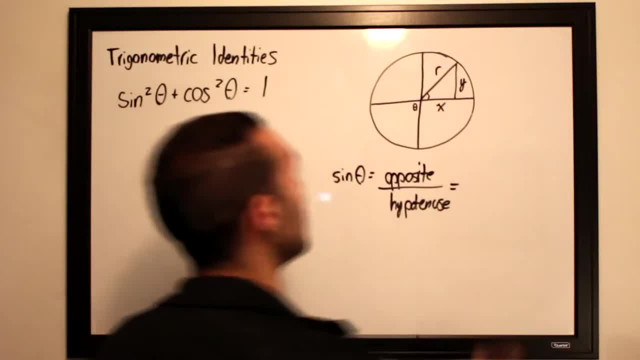 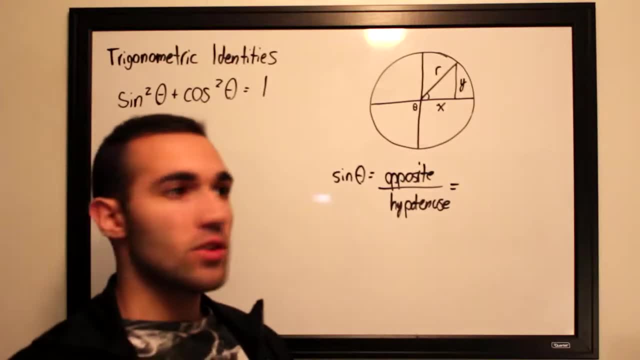 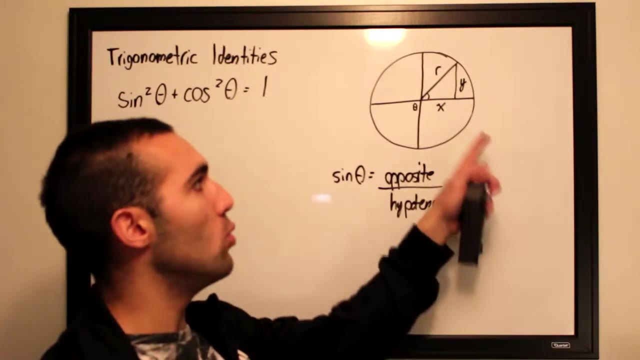 Here. we've got a unit circle right over here of radius r and we've got a triangle over here with length x and height y. So in terms of this triangle that we've got, which is part of the unit circle opposite, divided by hypotenuse, can also be viewed as y divided by hypotenuse. 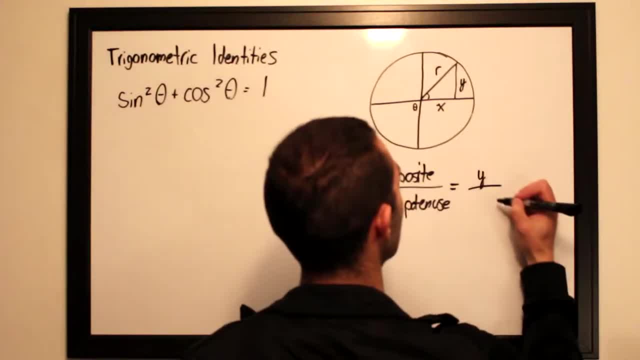 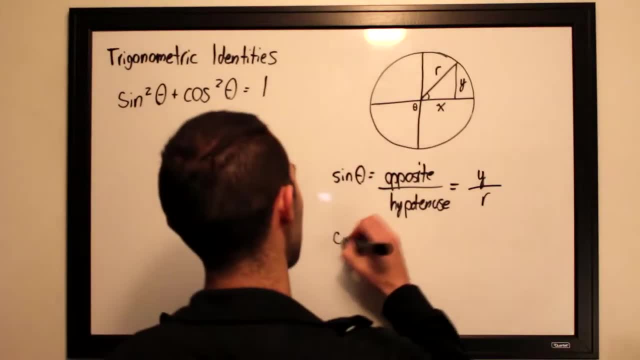 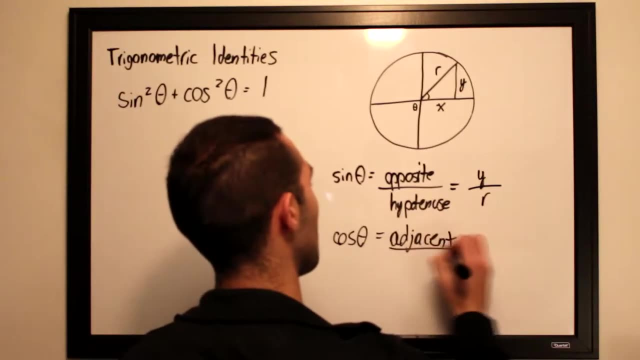 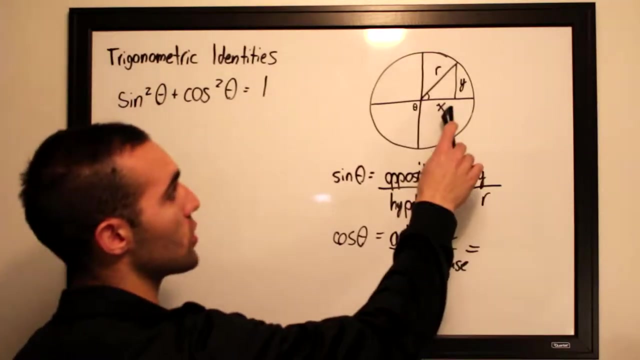 So the sine is actually the height of the function divided by the radius. Now we can do the same thing with the cosine. The cosine of theta is generally defined as the adjacent portion of the triangle divided by the hypotenuse, And according to this triangle, the cosine is going to be x divided by r. 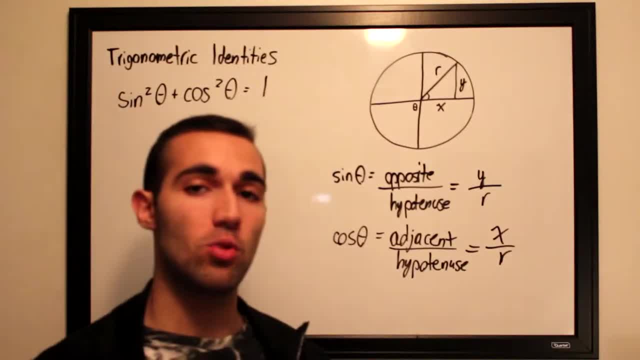 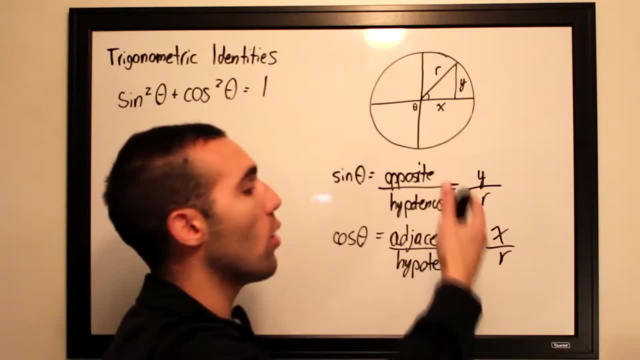 And now what I'd like to do is make a very simple equation. I'm going to use the Pythagorean theorem to solve for the equation of x squared plus y squared, divided by the hypotenuse of this triangle. So if we wanted to figure out what r was in terms of x and y, we can go ahead and solve for that using the Pythagorean theorem. 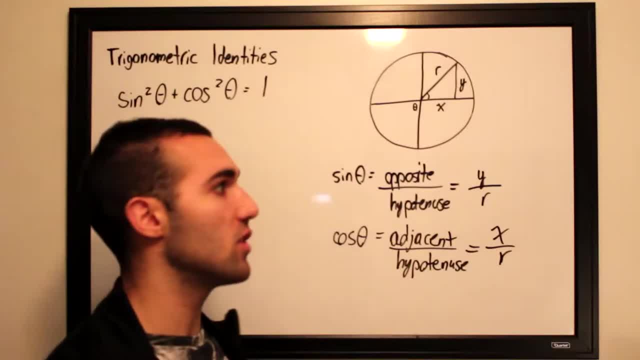 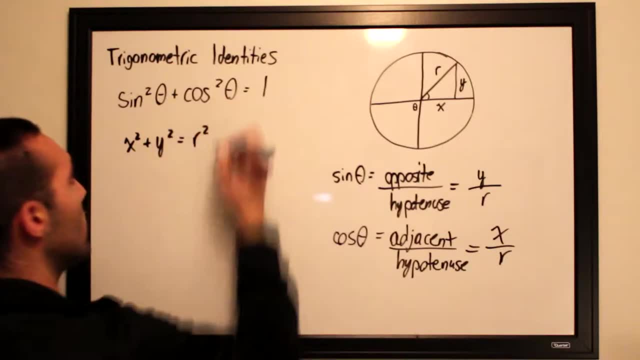 So essentially, what we can do is add up the square of both sides and then take the square root, where it is that x squared plus y squared is equal to r squared. This is just an application of the Pythagorean theorem: This squared plus this squared is equal to this squared. 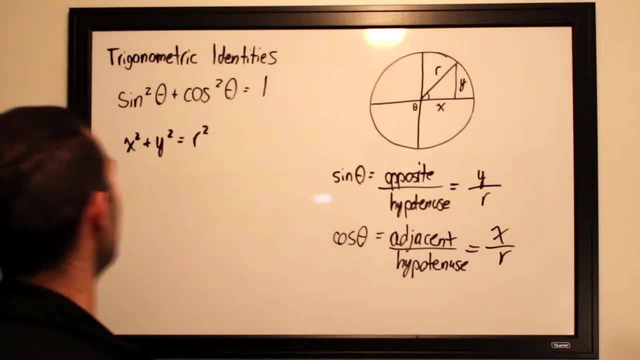 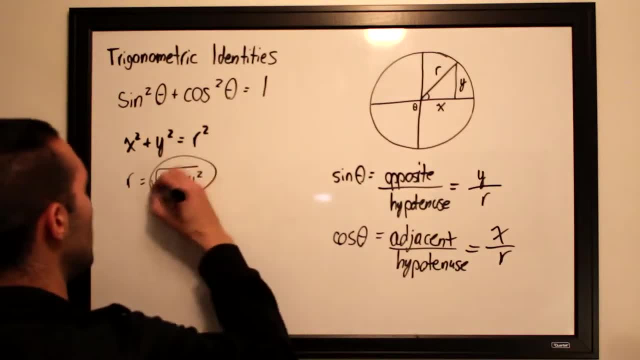 So if we wanted to isolate for r in terms of x and y, we can view r as the square root of x squared plus y squared. So we can go ahead and make that substitution for this portion over here and for this over here.